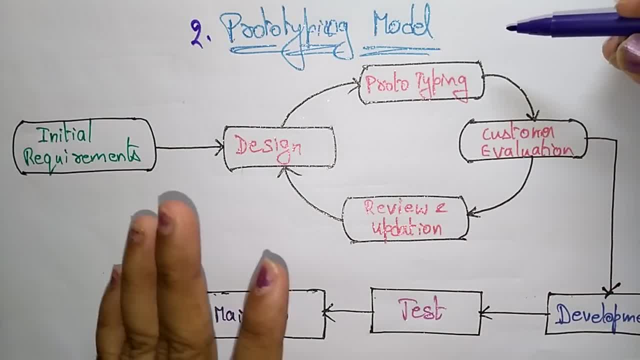 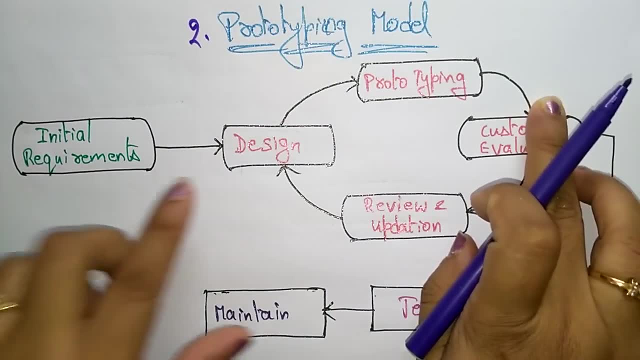 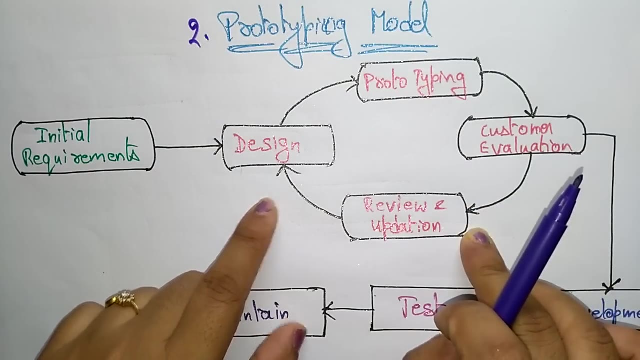 The prototyping means here it uses multiple iterations. We are doing this is a multiple iterations. That's why we are putting in this circle. So in prototyping model we use a multiple iterations or requirements, analysis and designs. So after each iteration the result is evaluated by the customer. So this is a problem here. means for every iteration means once: if you done the requirement phase, you have to. 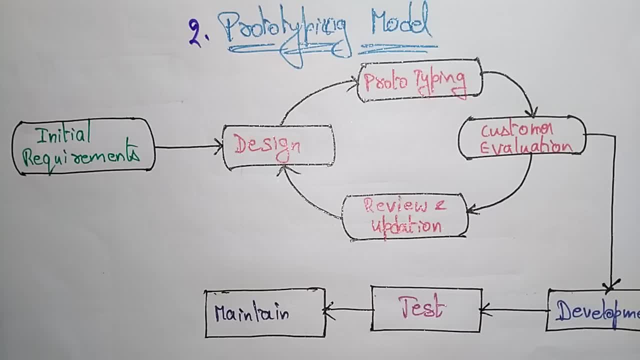 show to the customer. Once you done the analysis phase, you have to show to the customer and if he satisfied, you can continue. Once, if your design phase is over, you have to show to the customer Means the customer has to evaluated whenever he is supposed to, whenever he accepted, then only your proceed to the development phase. And here one more advantage is there, because once he satisfied, if you develop the product, if you write the code, then it will be. 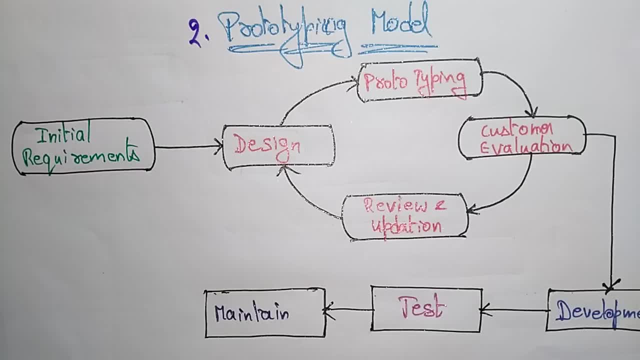 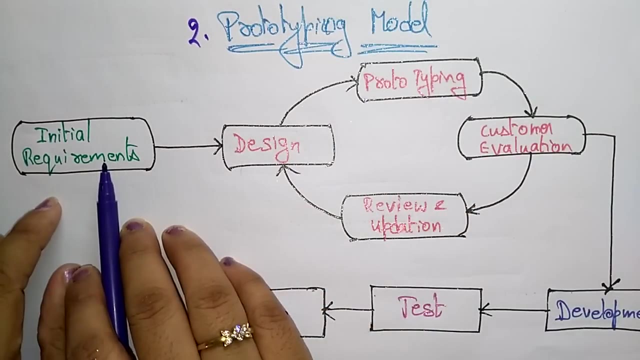 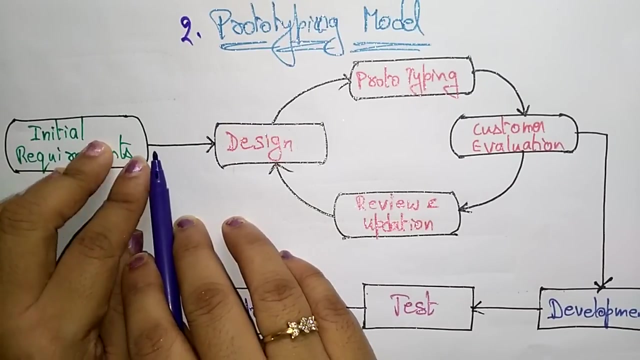 easy for us because once if you implemented the coding, also if the customer changes their requirement, it is difficult for the person who is developing the product because a burden will be increased. So that's why in prototyping model means it's just a- multiple iterations will be done here, So here. so first in the initial requirements, the customer will give the first initial requirements, whatever he wants. So whenever we take the initial requirement, we start the design. The team members will start the design. So after 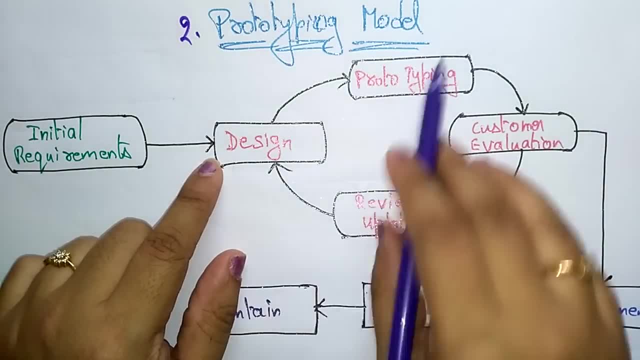 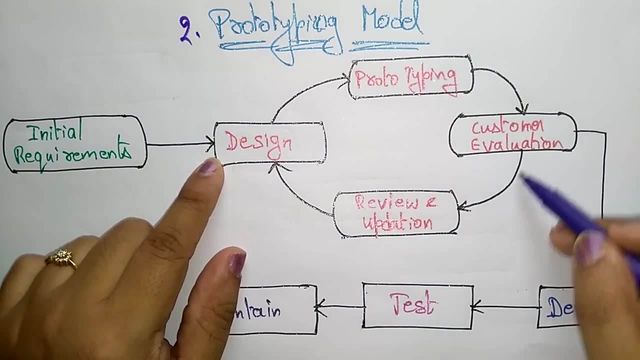 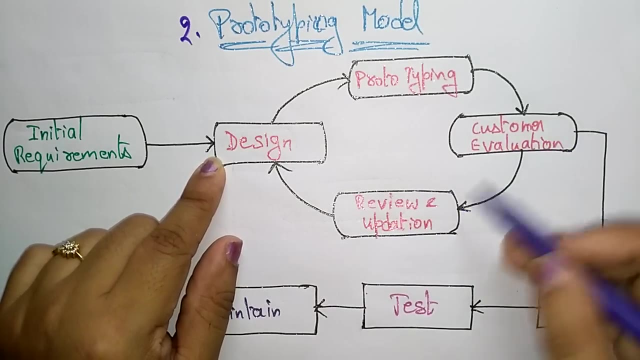 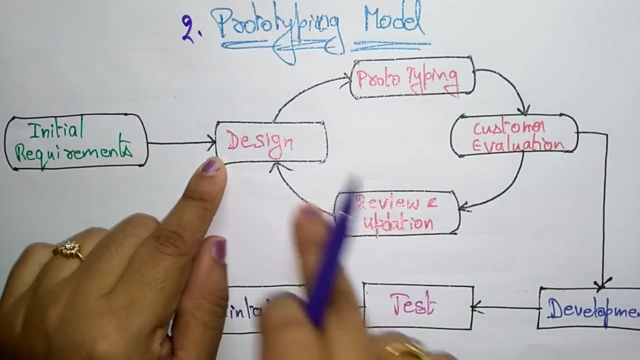 designing means they should the prototyping. Once he done the prototyping, they'll show to the customer. The customer has to evaluated. Okay, the customer is not satisfied. his review and updations means: I want some more to add to this product. I want to, I don't want like this. I just change that. like that, he is just evaluating the product. review and updations will be given by the customer. So again the persons will start the design, Then prototyping, Then the it give. 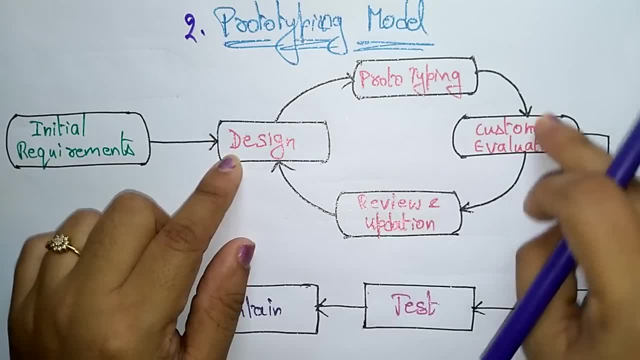 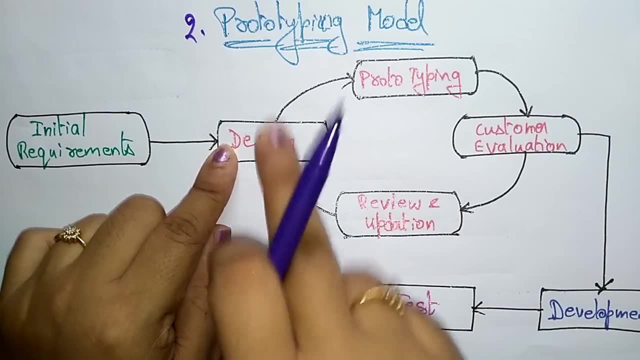 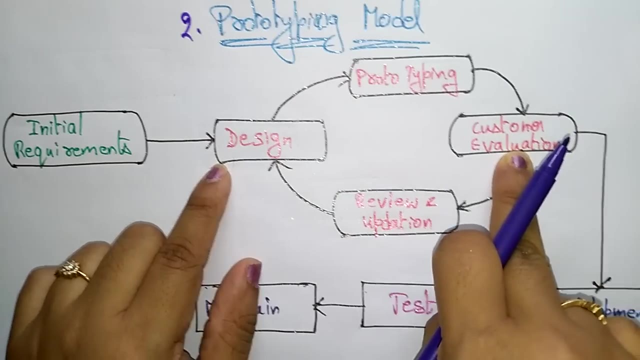 to the customer. okay, this time also the customer is not satisfied. again, review and updations. so whatever the review and updations that the customer is given, again they start the designing. so only their stage of this designing only. they are not started the implementation. so they design the product. so this time they satisfied. so, whenever they the initial requirements, 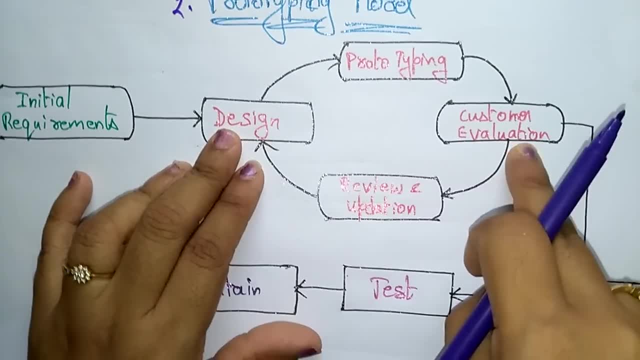 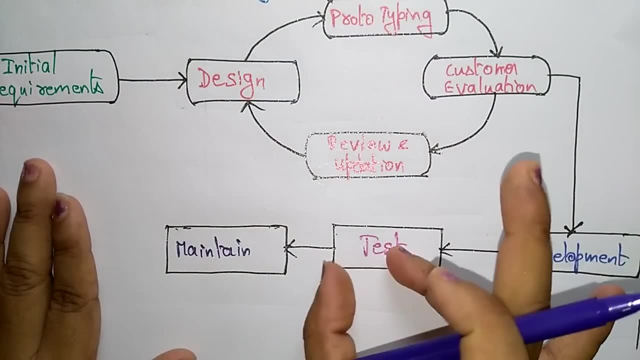 and the updations of the customers. everything is satisfied by the customer, then they will develop. the product means they implement the product by writing the code. so after writing the code they will test the product. then the test the product they will go for. the maintenance means they will. 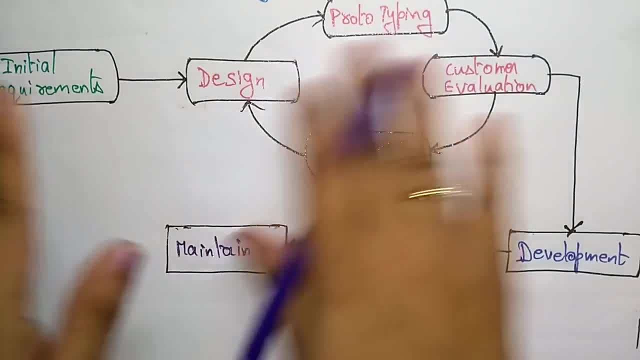 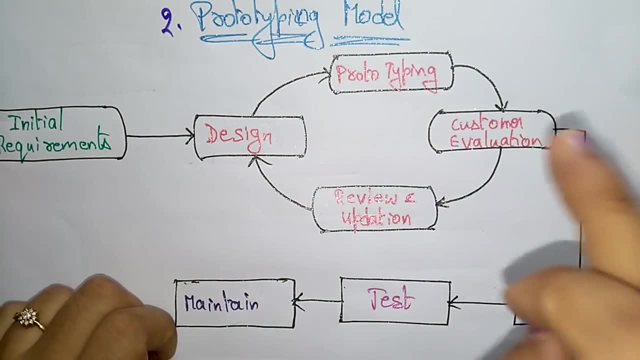 the. they will deliver the product and they will maintain the product. so this is how the prototyping model will be done. so after each iteration, the result is evaluated by the customer. so whenever this user is satisfied, the prototype code is brought up to the standards need for a final. 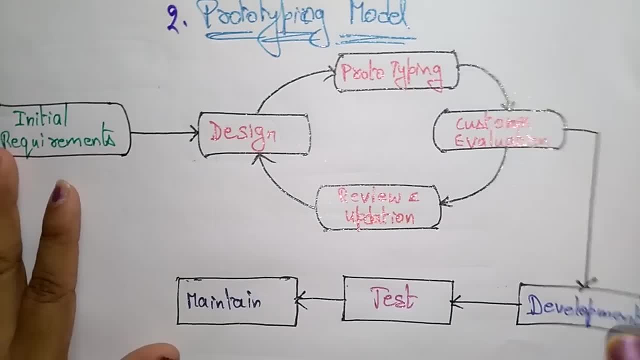 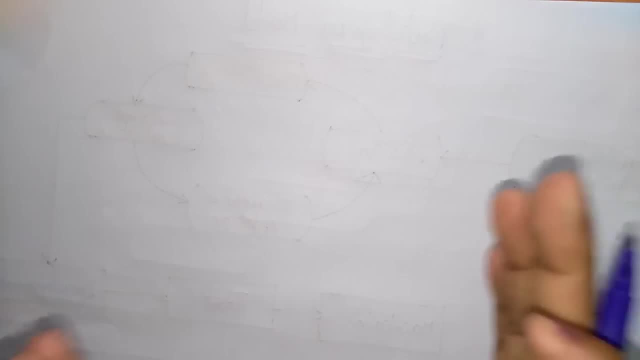 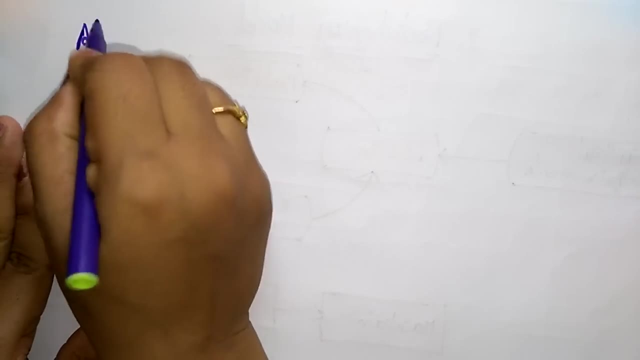 product. so this is about the prototyping model. now let us see the advantages and disadvantages. so actually everything, whatever you are taking, the models, everything, the software engineering, it should be present in diagram. so just you have to be elaborate that diagram. the advantages of prototyping model is customer can see steady 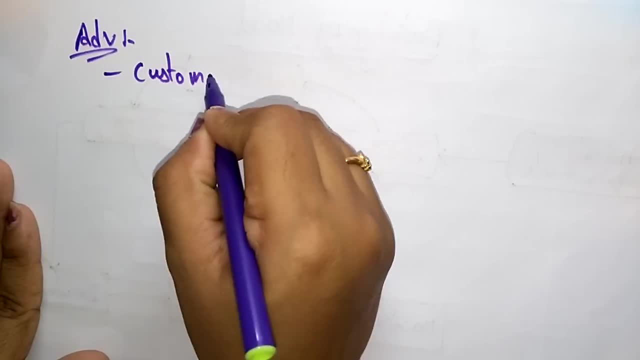 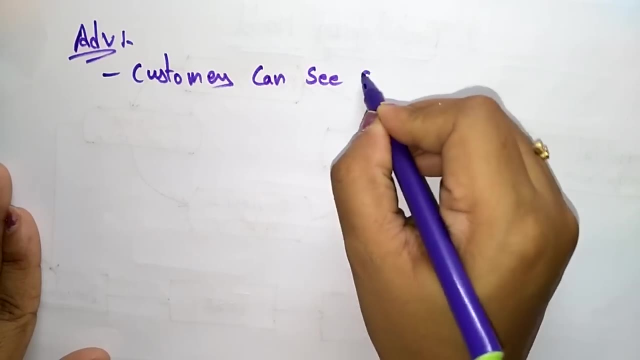 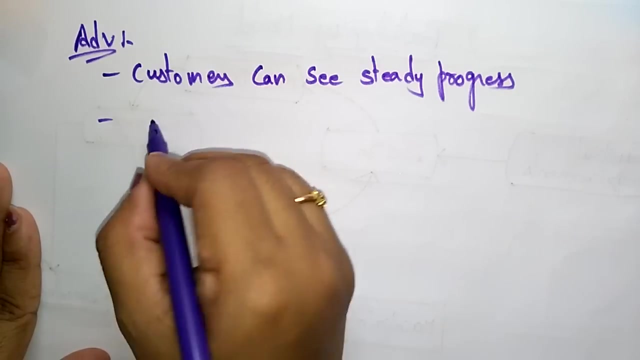 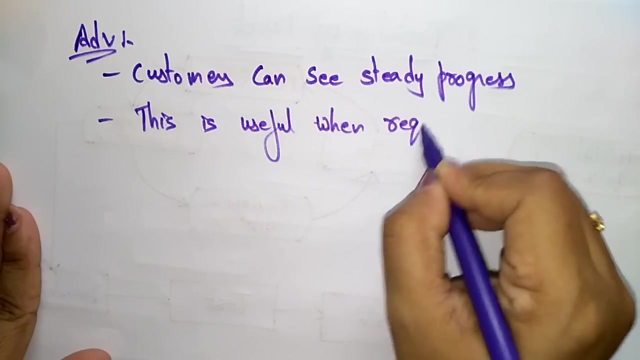 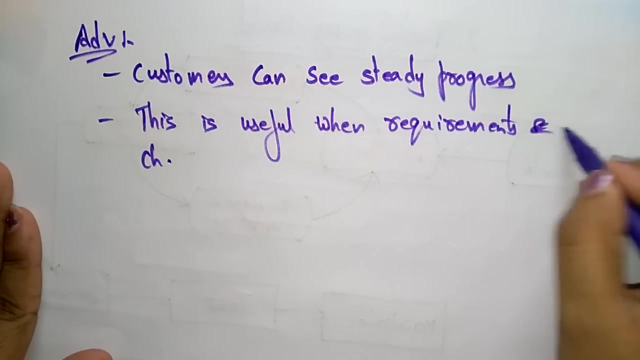 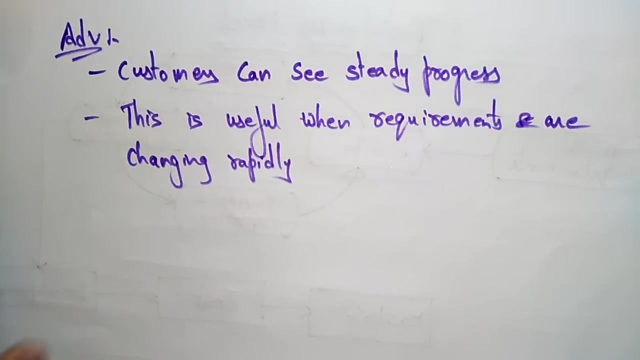 progress means in each stage they are seeing the progress of the product. customers can see a Steady progress. This is useful. This is useful when requirements aren't changing rapidly. So requirements are changing rapidly. So whenever the requirements are changing rapidly by the customer, if that customer is changing always he is if he changes. 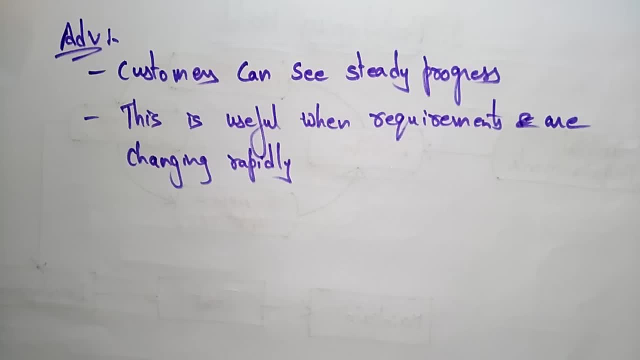 changing the his requirements, then it's better to go for the prototype model rather than going for the waterfall model. Waterfall model means once we started everything implementation, everything is testing, Once you deploy the product, then only the customer will check. If the customer didn't satisfied, again we have to be due. So that will be burden for the developers as well as the customers also. So it's better if the customer is rapidly changing. the decisions means then it's better to go for the prototype model.